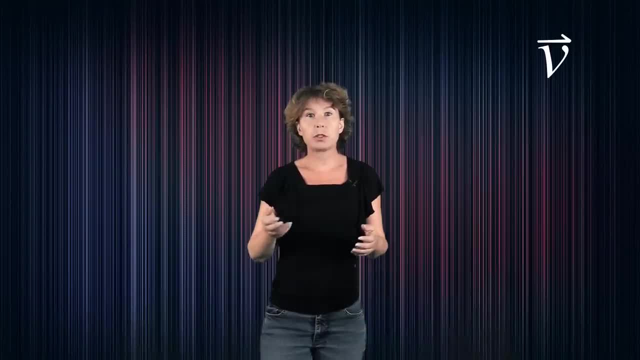 is important for understanding the assignment method and theWoodyí self. and Iv 무슨 difficult creates an official, invincible thing. It is known how to describe everything and how to operate. it is a vector just like the ones we learned about in school. 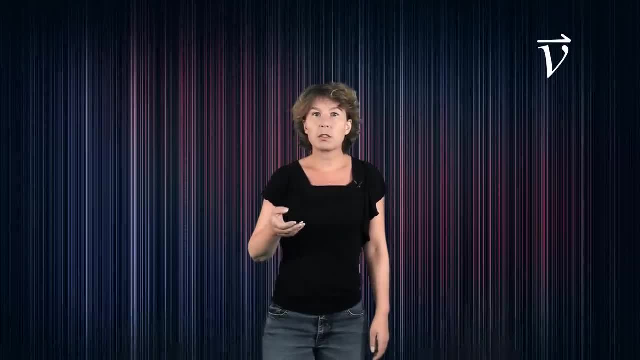 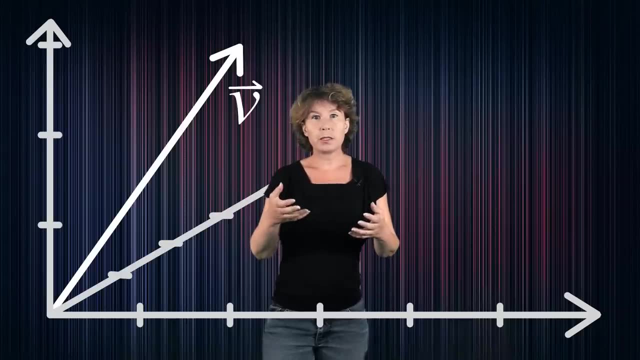 In a three-dimensional space. you can think of a vector as an arrow pointing from the origin of the coordinate system to any point. You can choose a particularly convenient basis in that space. typically, these are three orthogonal vectors, each with a length of one. 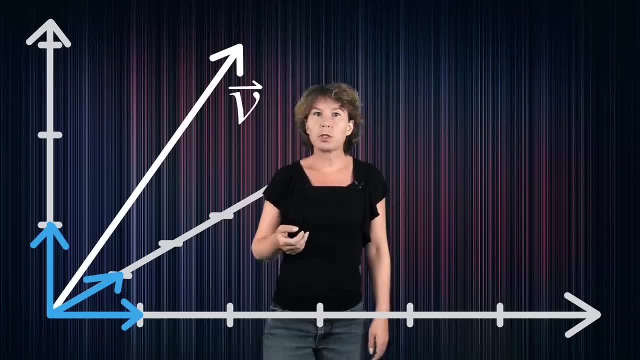 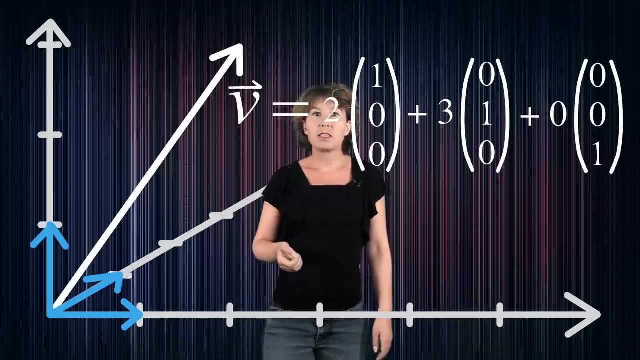 These basis vectors can be written as columns of numbers which each have one entry that equals one and all other entries equal to zero. You can then write an arbitrary vector as a sum of those basis vectors, with coefficients in front of them. say two, three, zero. 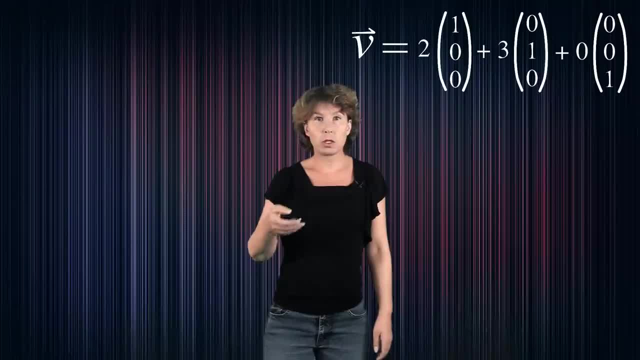 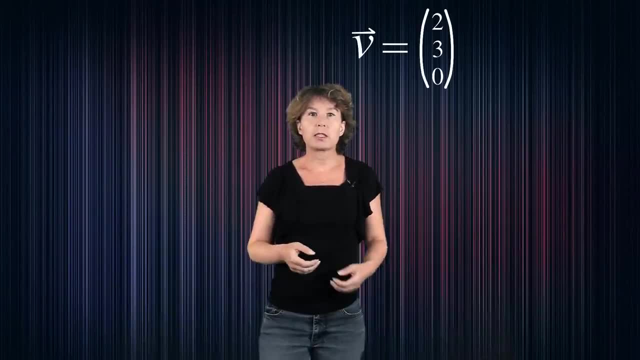 These coefficients are just numbers and you can collect them in one column. So far, so good. Now the wavefunction in quantum mechanics is a vector, just like that, except it's not a vector in the space we see around us, but a vector in an abstract mathematical thing. 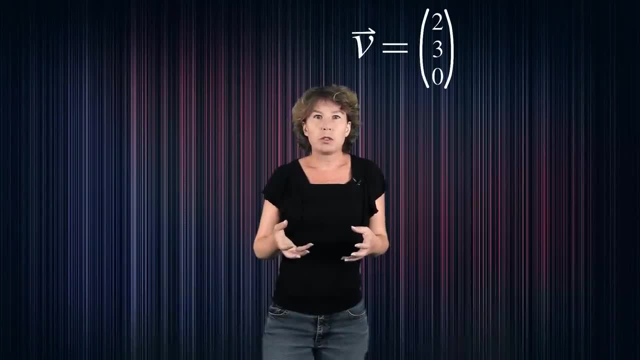 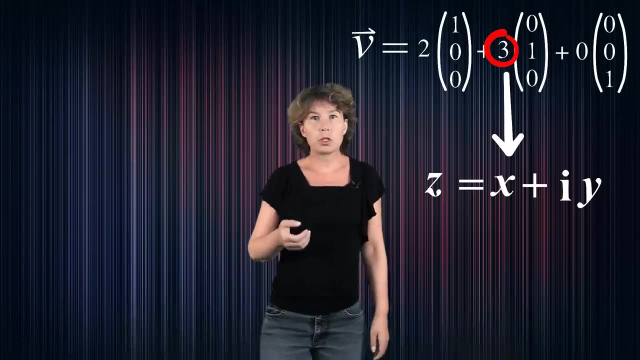 called a Hilbert space. One of the most important differences between the wavefunction and vectors that describe directions in space is that the coefficients in quantum mechanics are not real numbers, but they are complex numbers, so they in general have a non-zero imaginary part. 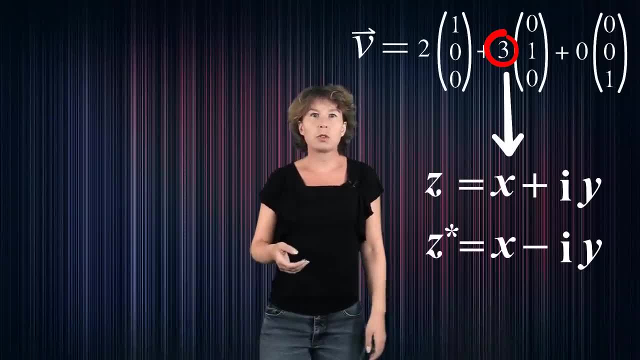 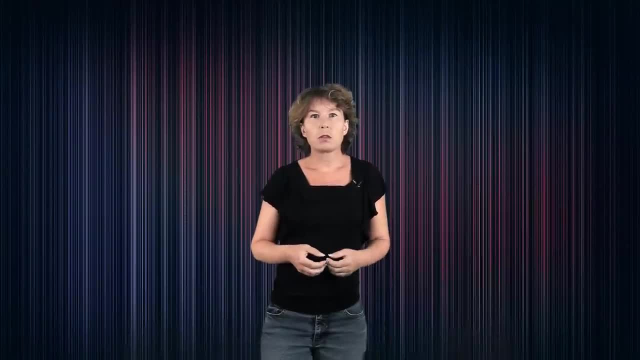 These complex numbers can be conjugated, which is usually denoted with a star superscript and just means you change the sign of the imaginary part. So These complex numbers make quantum mechanics different from your school math. But the biggest difference is really just the notation. 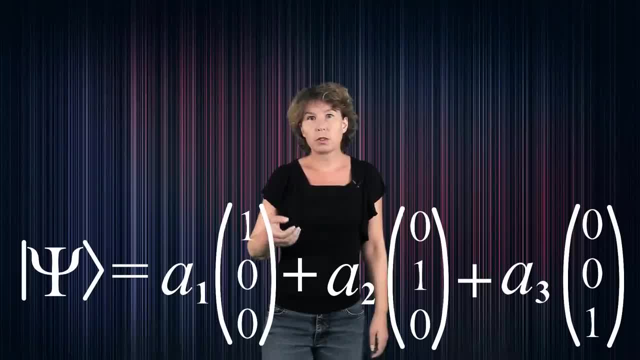 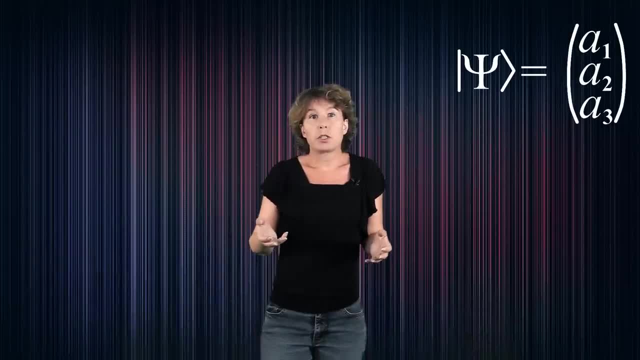 In quantum mechanics. we do not write vectors with arrows. Instead, we write them with these funny brackets. Why? Well, for one, because it's convention, But it's also a convenient way to keep track of whether a vector is a row or a column vector. 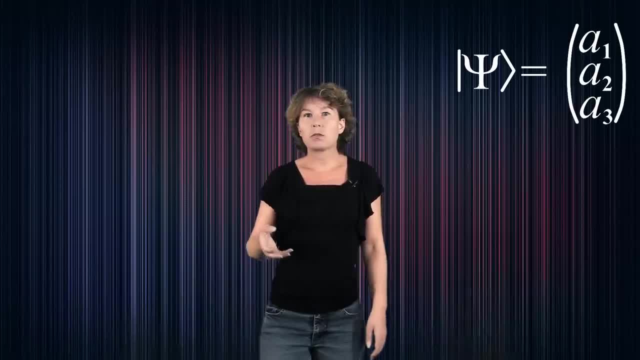 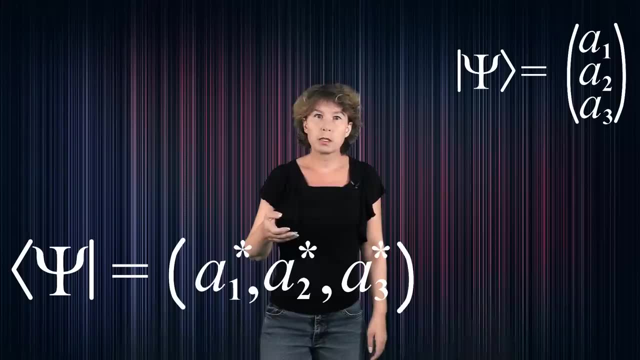 The ones we talked about so far are column vectors. If you have a row vector, instead you draw the bracket on the other side. You have to watch out here, because in quantum mechanics, if you convert a row vector to a column vector, you also have to take the complex conjugate of the coefficients. 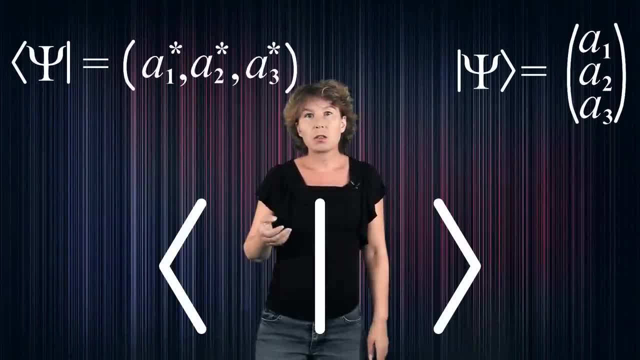 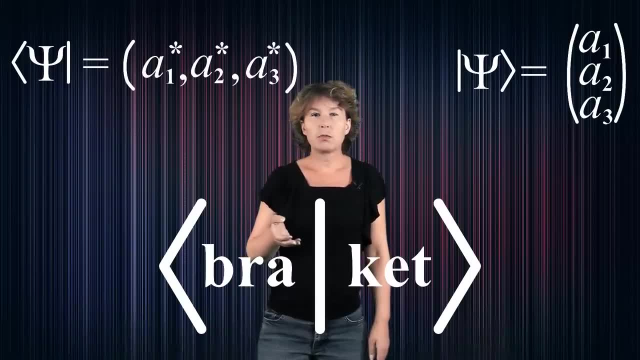 This notation was the idea of Paul Dirac and is called the bra-cat notation. The left side, the row vector is the bra and the right side, the column vector, is the cat. You can use this notation, for example, to write a scalar product conveniently as a bra-cat. 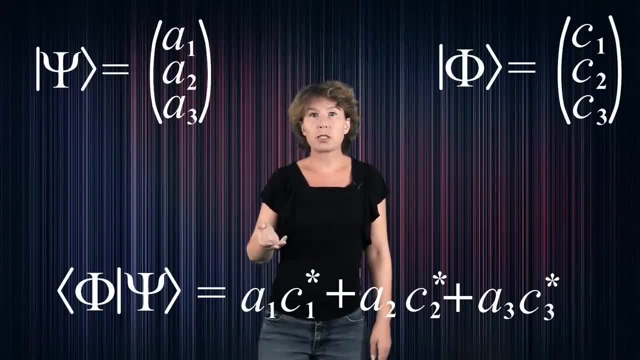 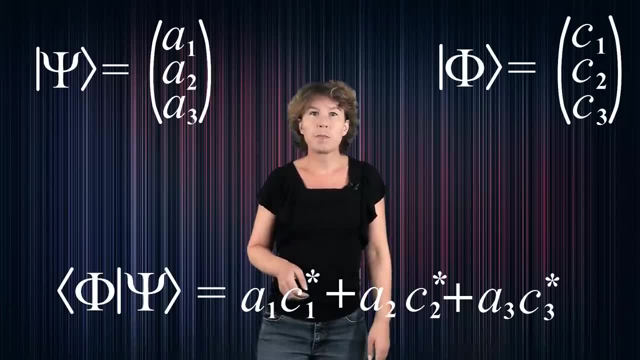 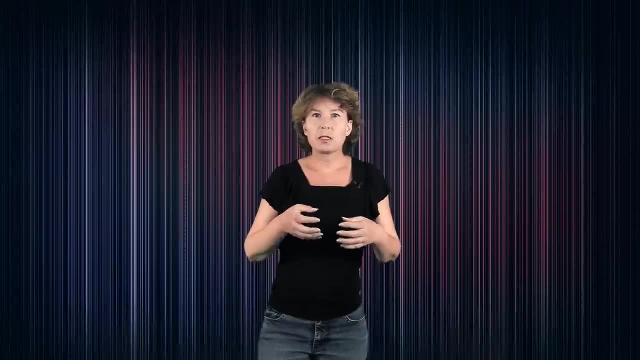 The scalar product between two vectors is the sum over the products of the coefficients. Again, don't forget that the bra vector has complex conjugates on the coefficients. Now, in quantum mechanics all the vectors describe probabilities And usually you choose the basis in your space so that the basis vectors correspond to possible. 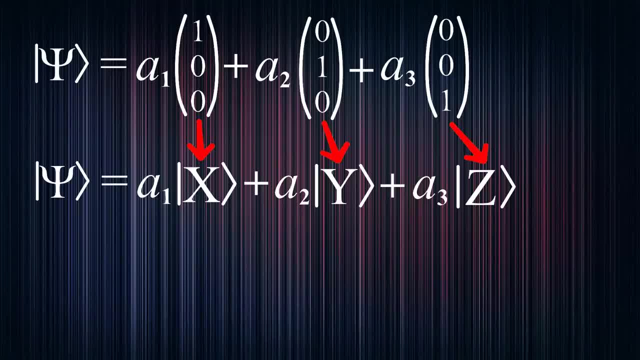 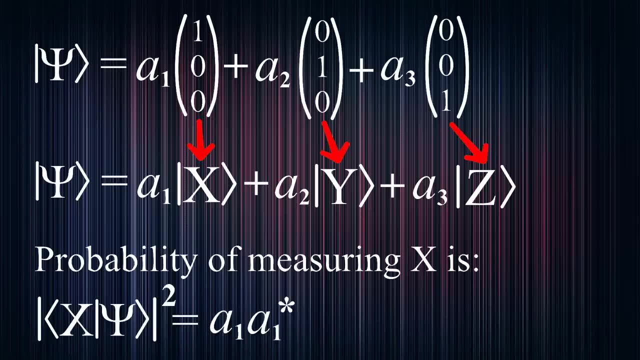 measurement outcomes. The probability of a particular measurement outcome is then the absolute square of the scalar product with the basis vector that corresponds to the outcome. Since the basis vectors are those which have only zero entries, except for one entry, which is equal to one, the scalar product of a wavefunction with a basis vector is just the coefficient. 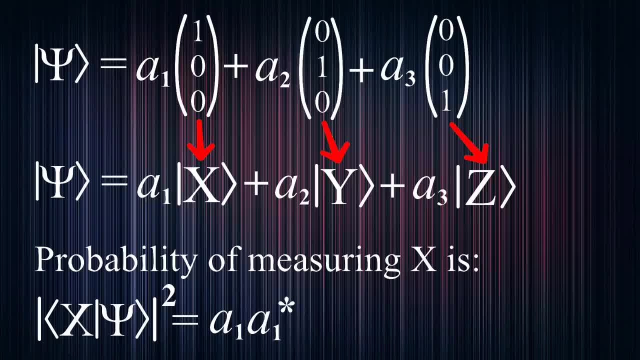 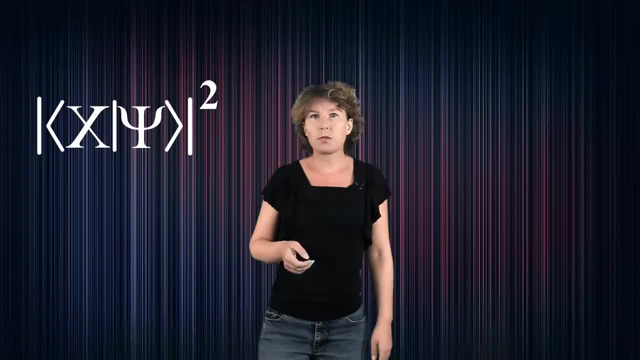 that corresponds to the one non-zero entry, And the probability is then the absolute square of that coefficient. So the probability of a particular measurement outcome is then the absolute square of the scalar product. This prescription for obtaining probabilities from the wavefunction is known as Born's. 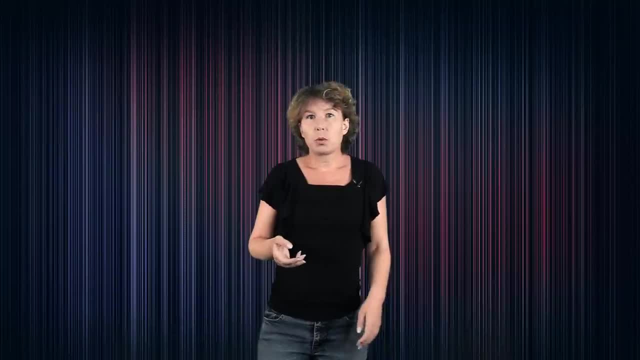 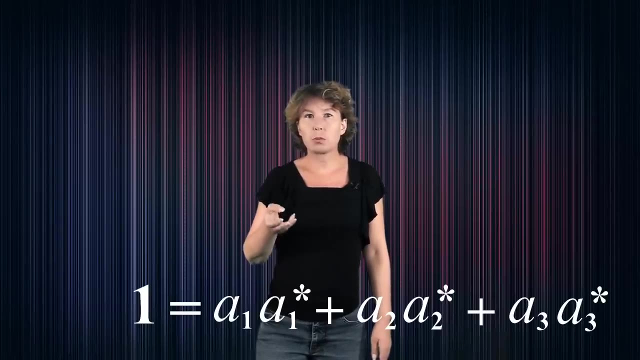 rule named after Max Born, And we know that the probability to get any measurement outcome is equal to one, which means that the sum over the squared scalar products with all basis vectors has to be one. But this is just the length of the vector. 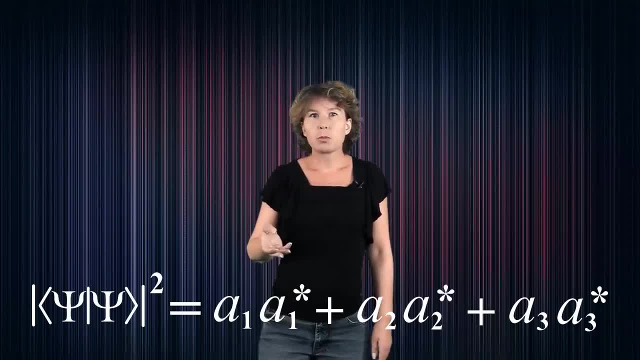 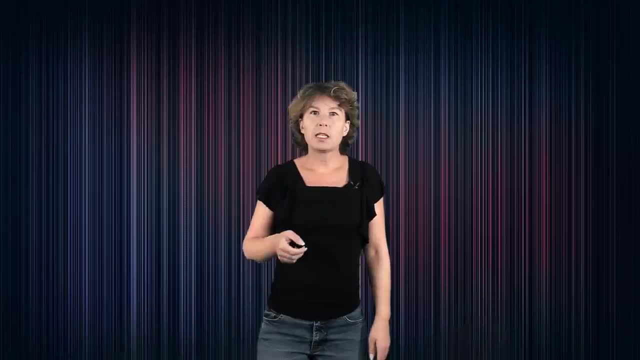 So all wavefunctions have length one. The scalar product of the wavefunction with a basis vector is also sometimes equal to one. This is sometimes called a projection on that basis vector. It is called a projection because it's the length you get if you project the full wavefunction. 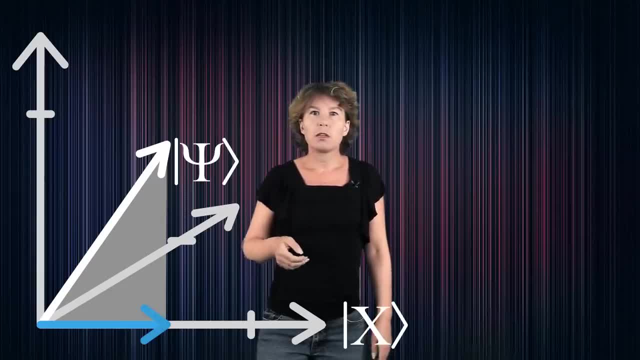 on the direction that corresponds to the basis vector. Think of it as the vector casting a shadow, You could say. in quantum mechanics we only ever observe shadows of the wavefunction. The whole issue with the measurement in quantum mechanics is now that once you do a measurement, 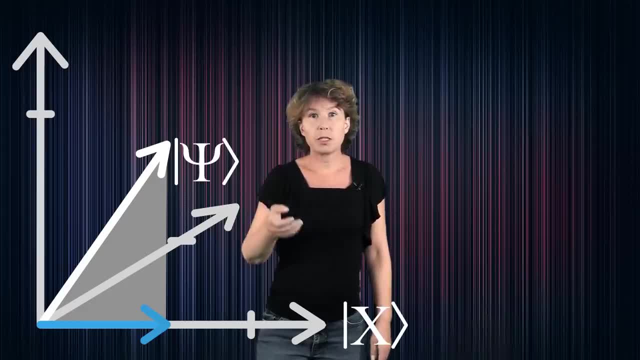 and you have projected the wavefunction. you can't measure it, So you can't measure it. If you are able to measure a wavefunction on to one of the basis vectors, then its length will no longer be equal to one, Because the probability of getting this particular measurement outcome may have been smaller. 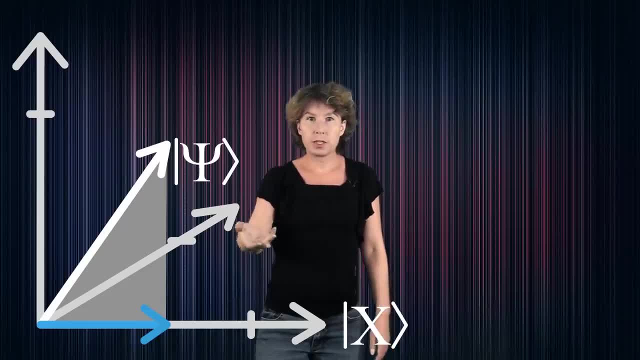 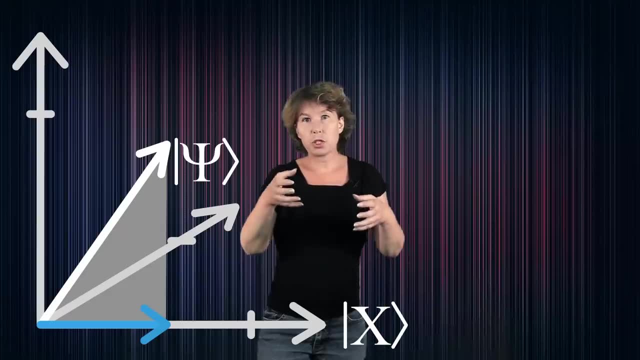 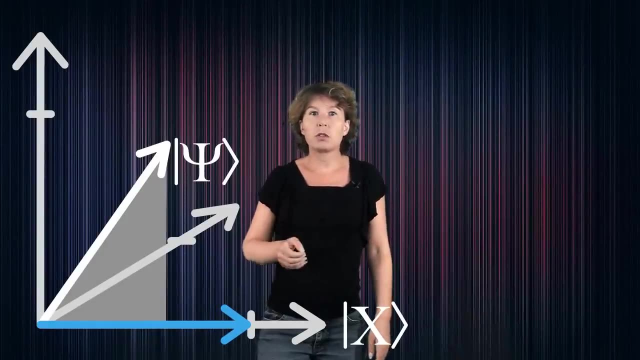 than one. But once you have measured the state, it is, with probability 1, in one of the basis states. So then you have to choose the measurement outcome that you actually found and stretch the length of the vector back to one. This is what is called the measurement update. 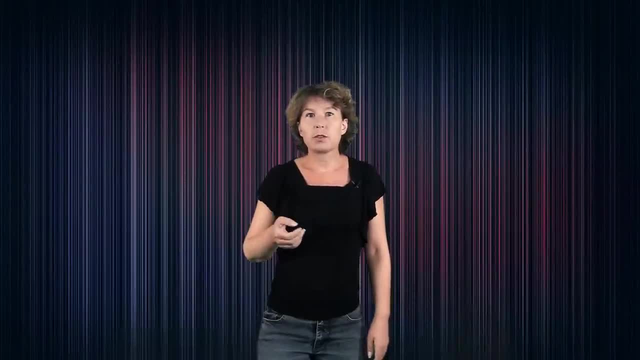 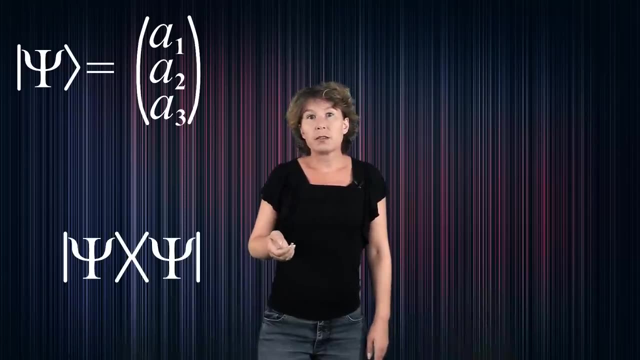 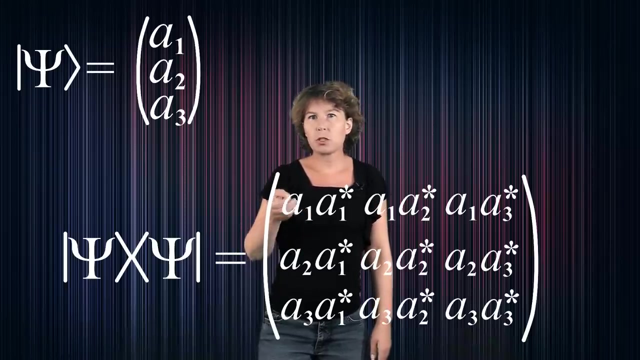 See you soon. Another thing you can do with these vectors is to multiply one with itself the other way around, so that would be a cat bra. What you get then is not a single number, as you would get with the scalar product, but a matrix, each element of which is a product of coefficients of the vectors. 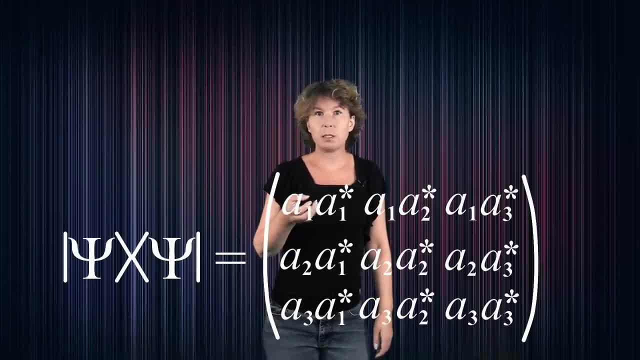 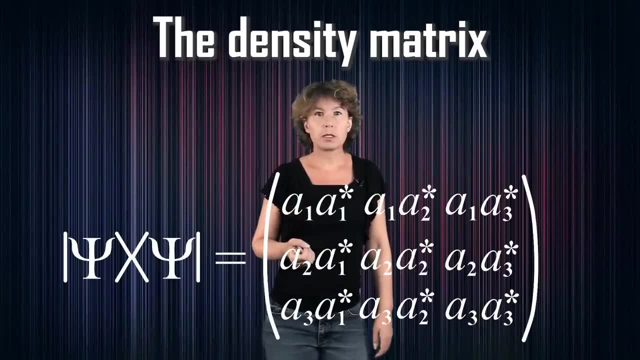 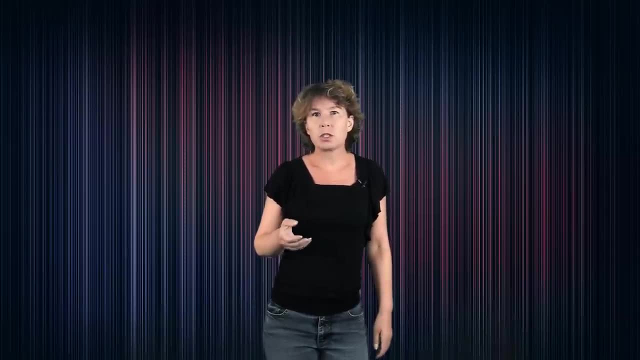 In quantum mechanics. this thing is called the density matrix and you need it to understand decoherence. We will talk about this some other time, so keep the density matrix in mind. Having said that, as much as I love doing these videos, if you really want to understand quantum, 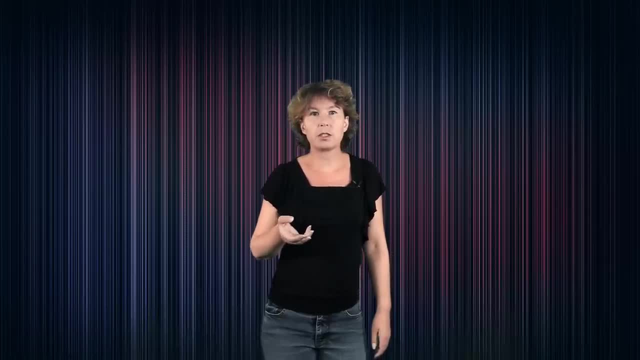 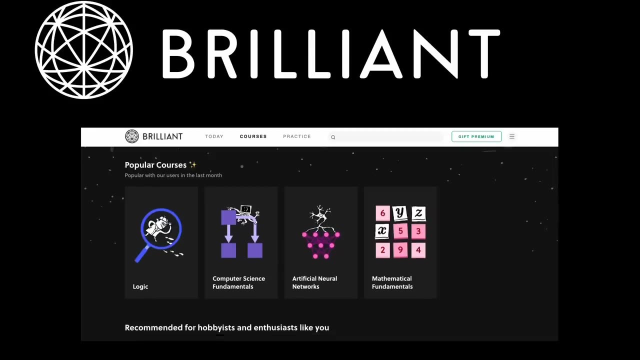 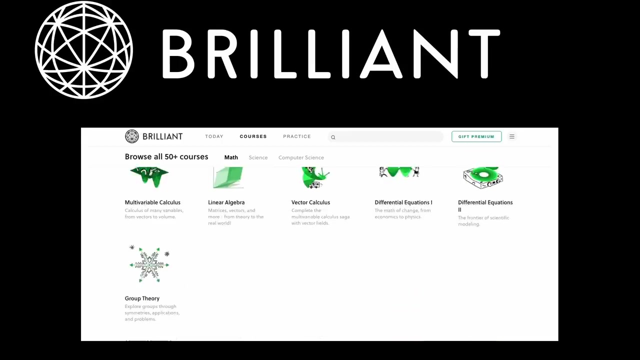 mechanics. you have to do some mathematical exercises on your own. A great place to do this is Brilliant, who have been sponsoring this video. Brilliant offers courses with exercise sets on a large variety of topics in science and mathematics. It's exactly what you need to move from passively 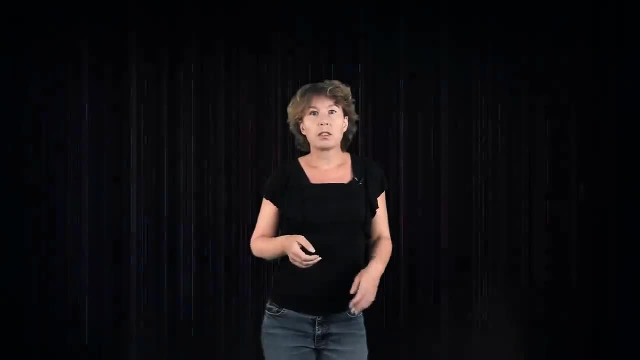 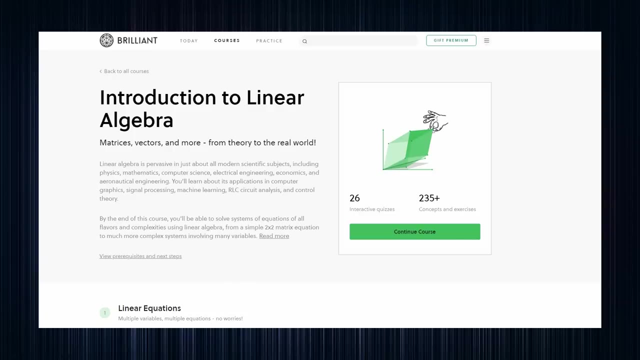 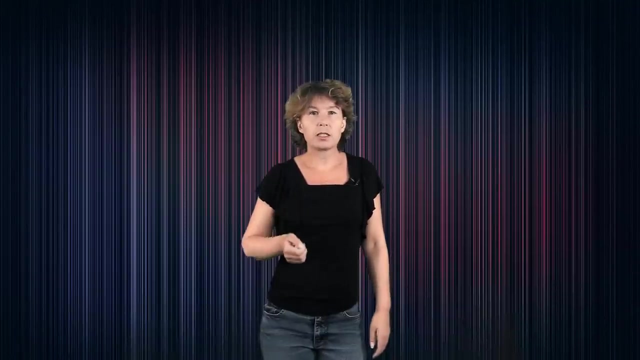 watching videos to actively dealing with the system. The courses on Brilliant that will give you the required background for this video are those on linear algebra and its applications. What is a vector? What is a matrix? What is an eigenvalue? What is a linear transformation? That's the key to understanding quantum mechanics. 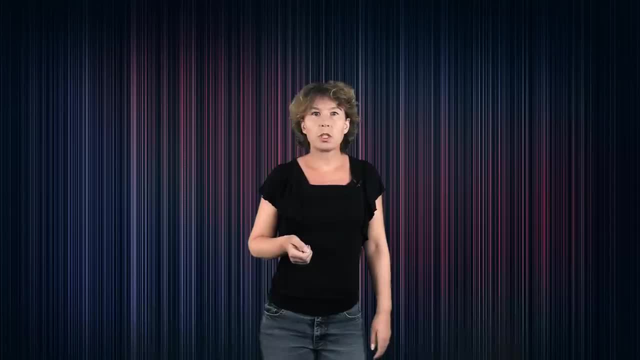 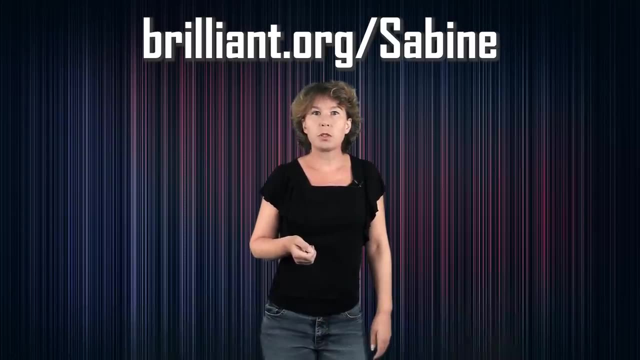 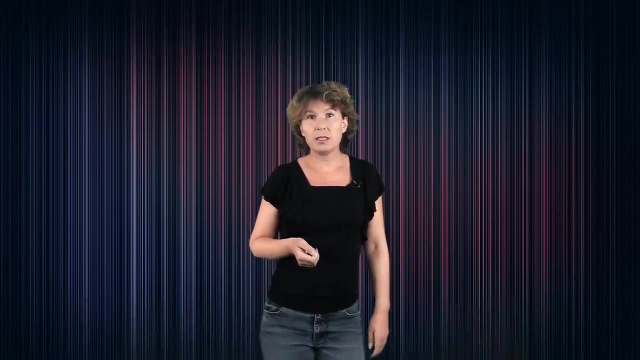 To support this channel and learn more about Brilliant, go to brilliant dot org. slash sabine- that's s-a-b-i-n-e- and sign up for free. The first 200 people who go to that link will get 20% off the annual premium subscription. You may think I made it look too easy, but it's true. 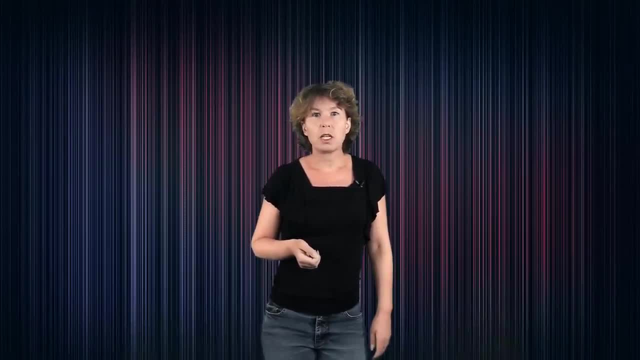 Quantum mechanics is pretty much just linear algebra. What makes it difficult is not the mathematics. What makes it difficult is how to interpret the mathematics. The trouble is you cannot directly observe the wave function. But you cannot just get rid of it either. 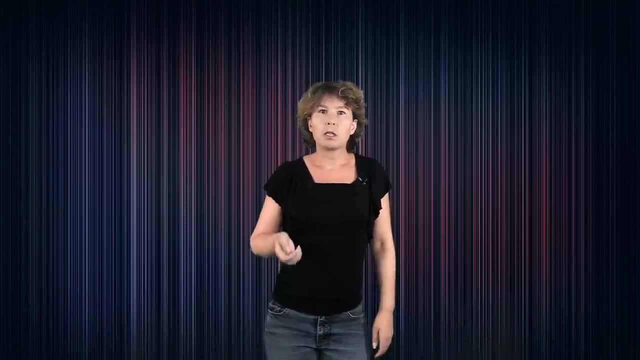 You need it to calculate probabilities, But the measurement update has to be done instantaneously And therefore it does not seem to be a physical process. So is the wave function real, or is it not? Physicists have debated this back and forth for more than 100 years.